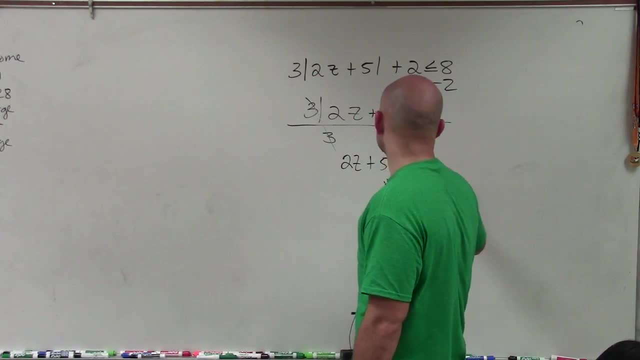 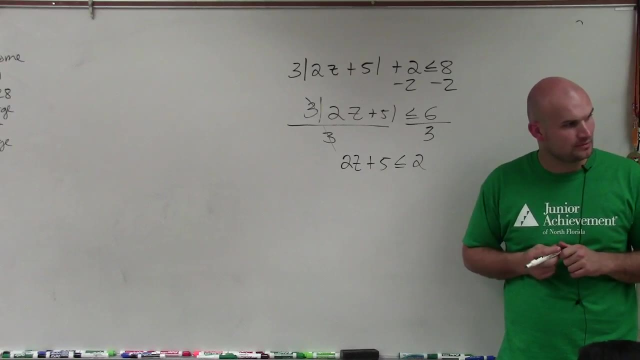 I'm left with 2z plus 5 is less than or equal to 2.. Oh okay, I'm sorry. Did I lose you on something? How did I do what, Huh? I divided 6, divided by 3, which was 2.. 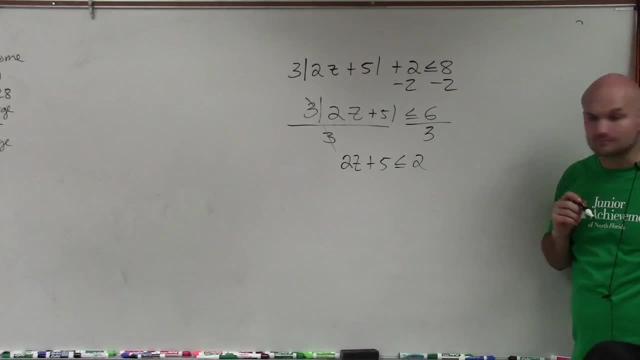 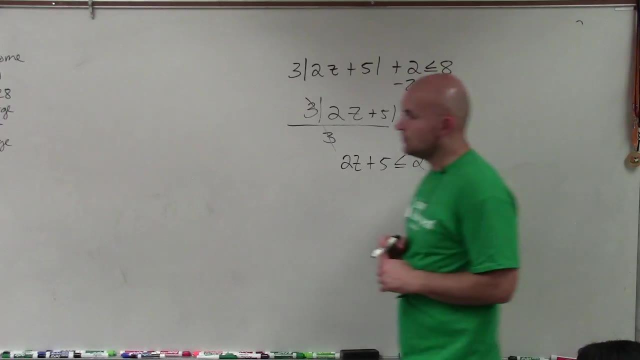 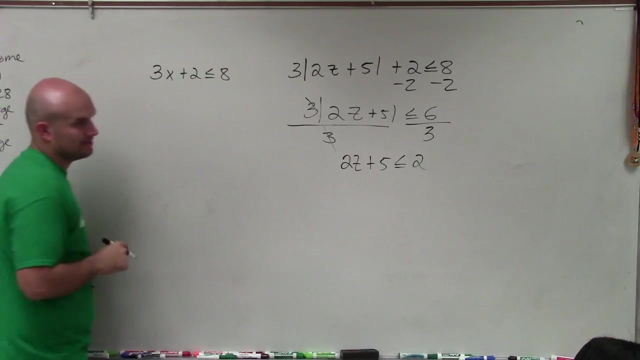 You're solving an equation like this. 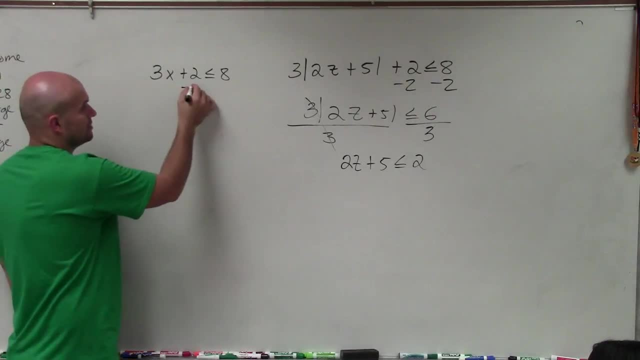 The first thing we need to do is undo addition and subtraction. Now, the next thing we need to do is undo multiplication, So we divide by 3.. Now, this is the exact same thing, except for this problem We had: x was equal to the absolute value of 2z plus 5.. 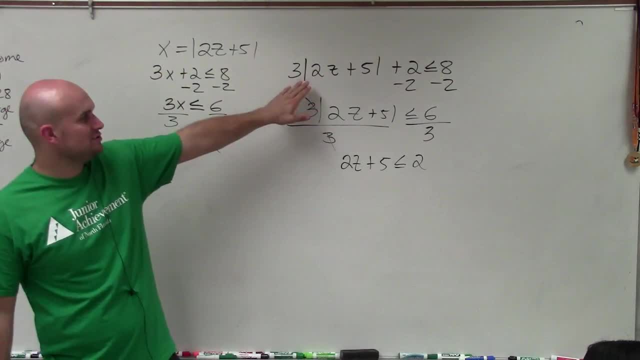 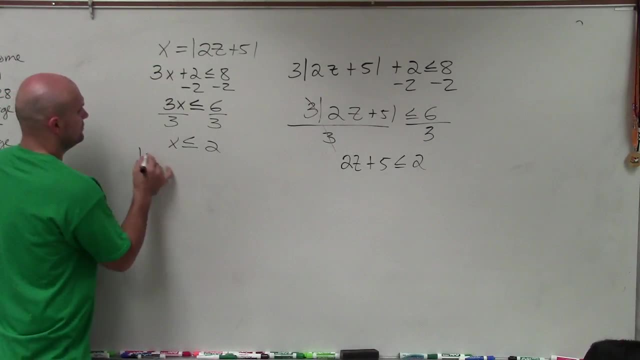 So if you'd rather rewrite the absolute value of 2z plus 5 as a variable x, that's perfectly fine, And then, since you know x is equal to that, you can plug it just back in at the end. Yes, Brandon. 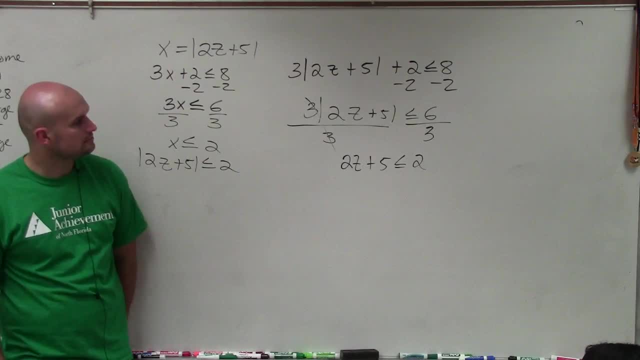 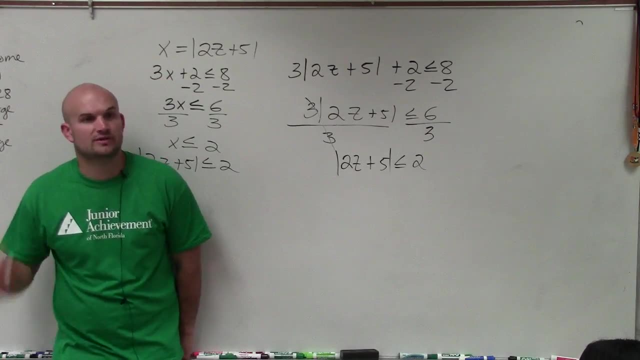 Why didn't you drop the empty line? I didn't. It's still supposed to be there, But does anybody have any general questions? Sinan, I'll give you one more chance and then I'm taking the phone. OK, I'm just telling you. 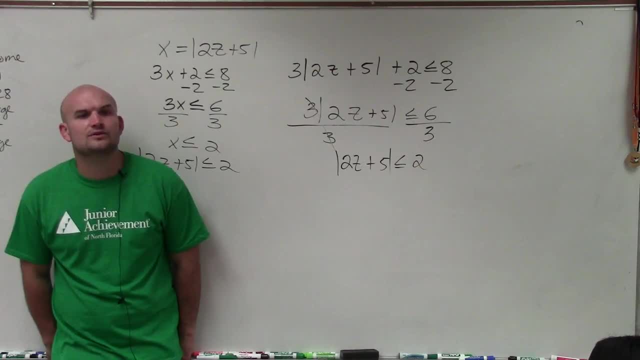 It really doesn't matter. So does anybody have any other questions? Because I think I've been very, very fair with you. You've actually been way too fair. Yes, Are you supposed to keep drawing after? Yeah, we're not done. 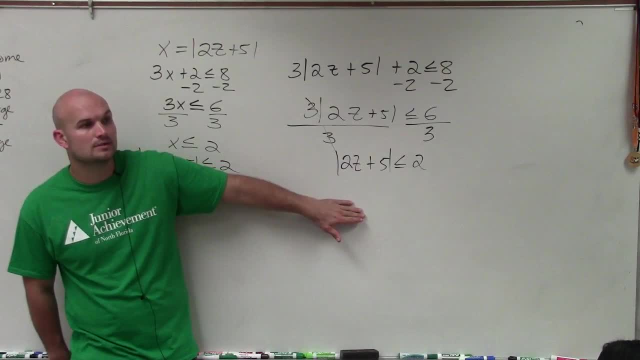 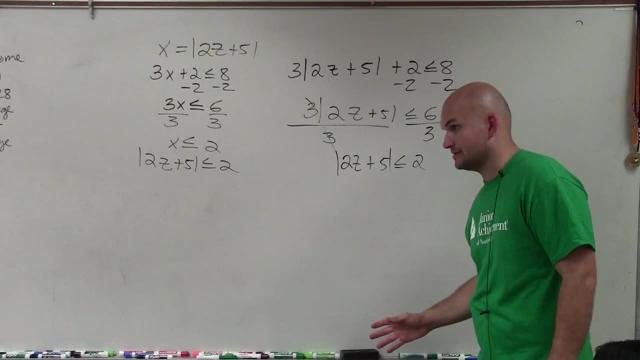 I'm just saying: does anybody have any questions up to this point? Does anybody have any questions up to this point? OK, what's your question? So you don't have a question? That's not a question. I don't want to erase that one. 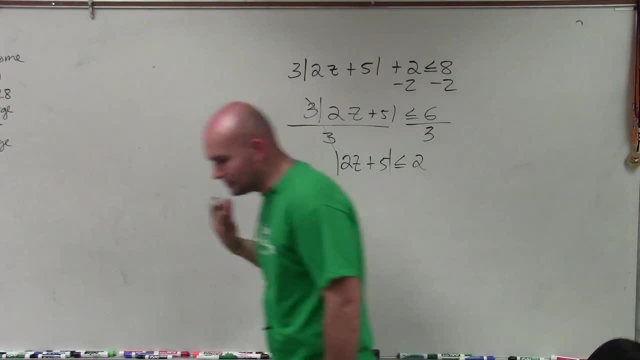 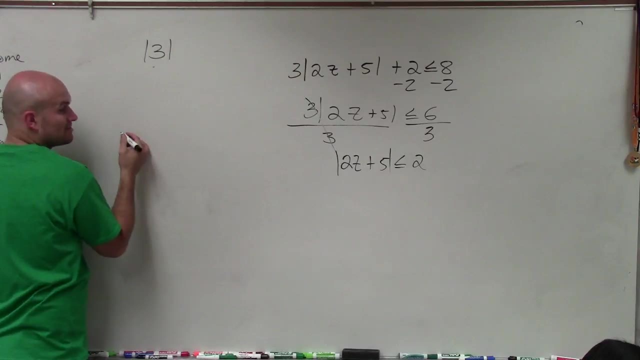 OK. So the next thing, ladies and gentlemen, is we've got to understand What exactly is the absolute value equation represented as a mean. So let's go back. through. what exactly does the absolute value represent? Remember, the absolute value represents the distance. 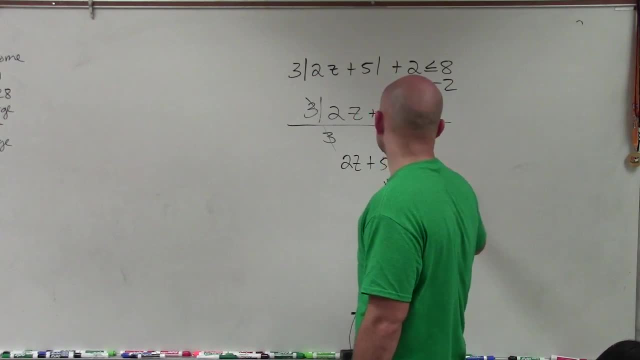 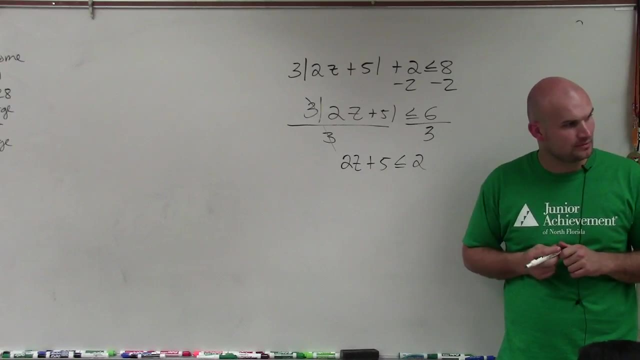 I'm left with 2z plus 5 is less than or equal to 2.. Did I lose you on something? How did I do what? Huh, I divided 6, divided by 3, which was 2.. Wait, so you can do another one and go a little slower, Or like, redo one, or 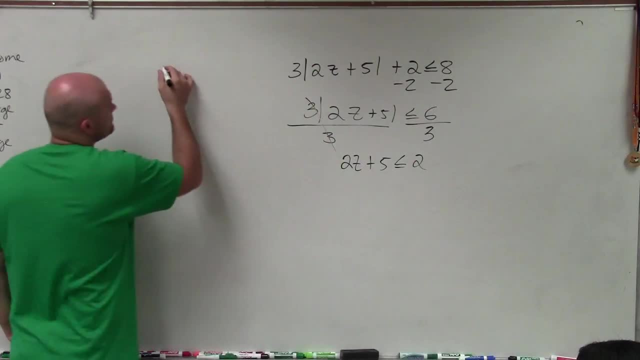 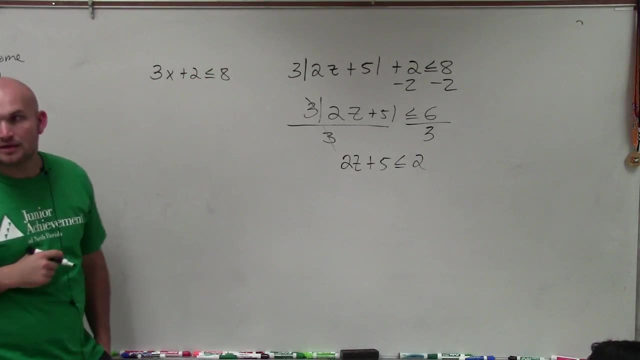 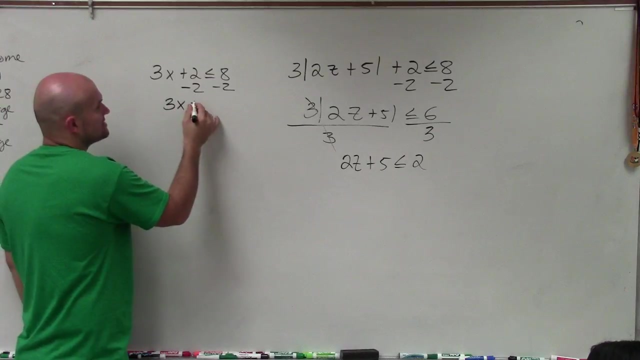 Okay, So Think about it this way You're solving an equation like this. The first thing we need to do is undo addition and subtraction. Now, the next thing we need to do is undo multiplication, So we divide by 3.. 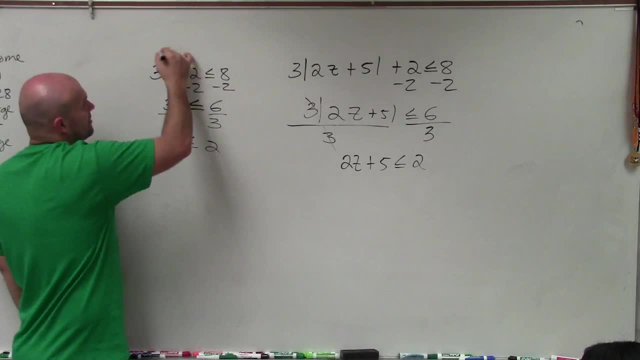 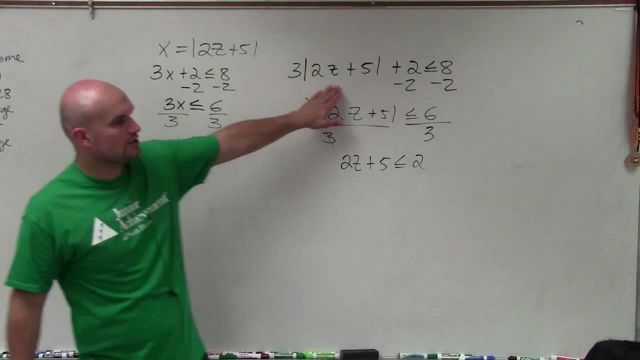 Now, this is the exact same thing, except for this problem We had x was equal to the absolute value of 2z plus 5.. So if you'd rather rewrite the absolute value of 2z plus 5 as a variable x, that's perfectly fine. 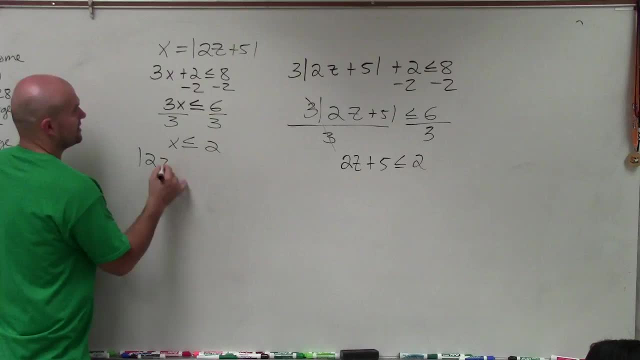 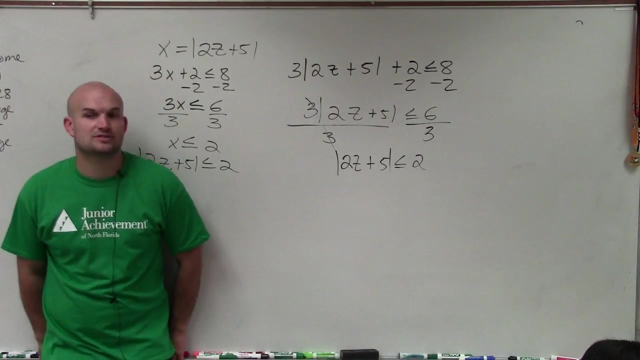 And then, since you know x is equal to that, you can plug it just back in at the end. Yes, Brandon, Why didn't you drop the empty line? I didn't. It's still supposed to be there. But does anybody have any general questions? 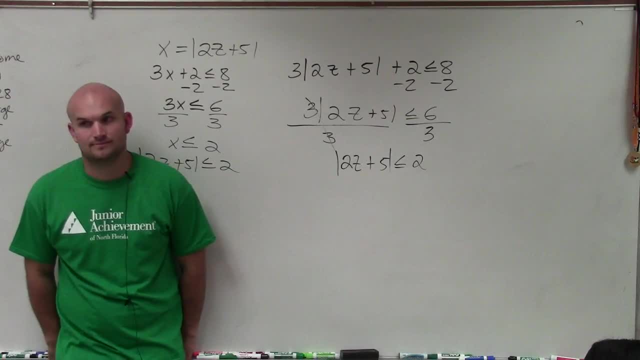 Sinan, I'll give you one more chance and then I'm taking the phone. OK, I'm just telling you, It really doesn't matter. So does anybody have any other questions? Because I think I've been very, very fair with you. 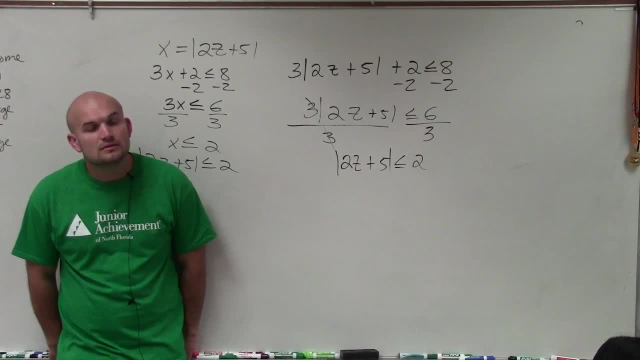 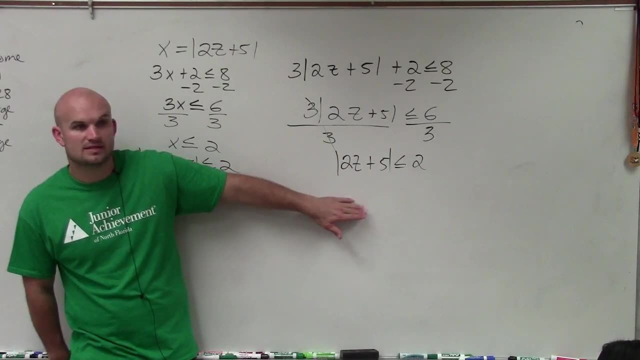 You've actually been way too fair. Yes, Are you supposed to keep drawing after? Yeah, we're not done. I'm just saying: does anybody have any questions up to this point? Does anybody have any questions up to this point? OK, what's your question? 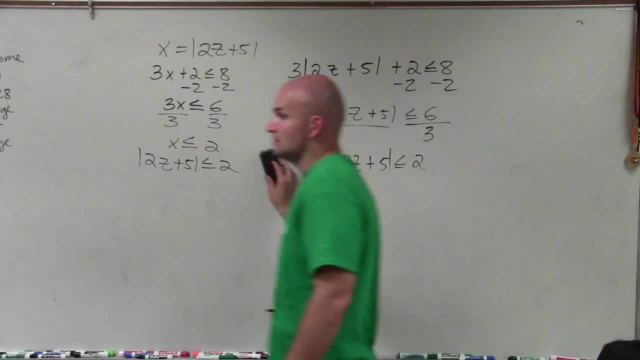 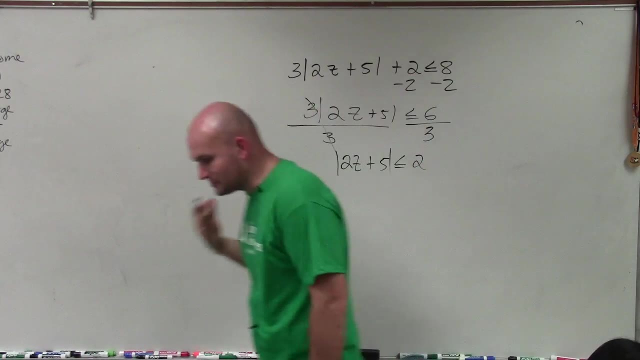 So you don't have a question. That's not a question. I don't want to erase that one. OK, So the next thing, ladies and gentlemen, is we've got to understand What exactly is the absolute value equation represented as a mean. 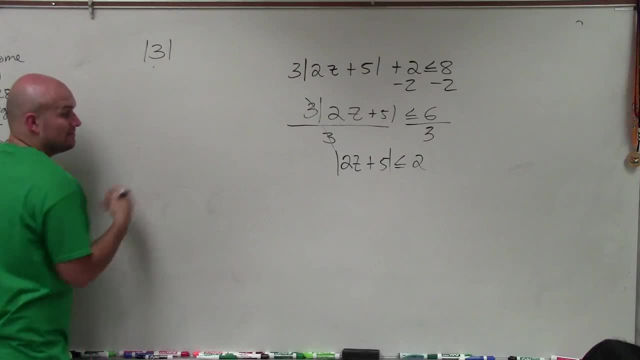 So let's go back through. what exactly does the absolute value represent? Remember, the absolute value represents the distance, Kaylee, from 0. So the absolute value is 3.. Absolute value of negative 3 is equal to positive 3.. 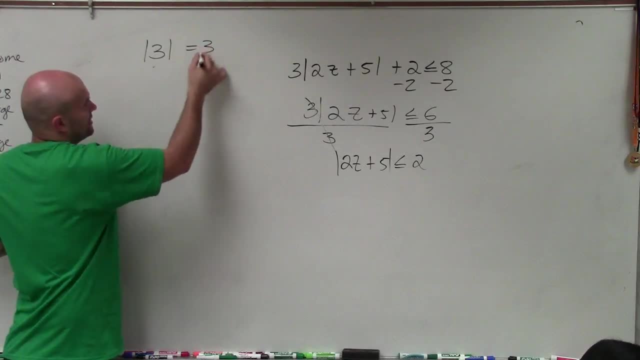 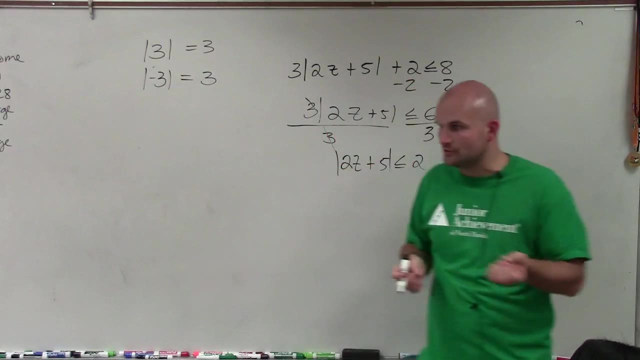 Kaylee, from 0. So the absolute value is 3.. Absolute value of negative 3 is equal to positive 3.. So the absolute distance is always that positive value, or the positive distance from, or just the distance from 0,, like when. 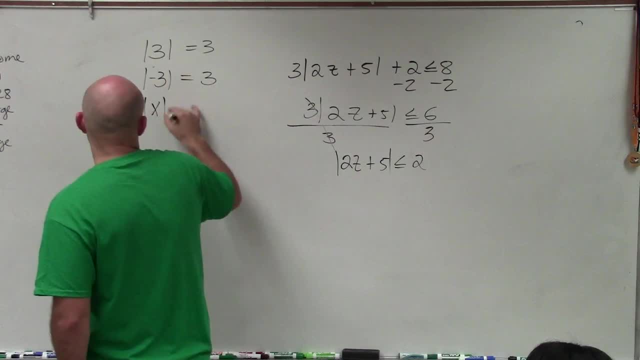 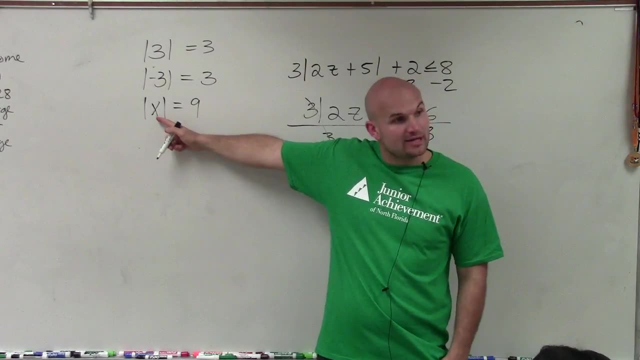 you look at the number line. So if I said the absolute value of x is equal to 9,, hopefully you guys can understand that I could plug in negative 9 in for x, or I can plug in positive 9,, correct? Does that make sense? 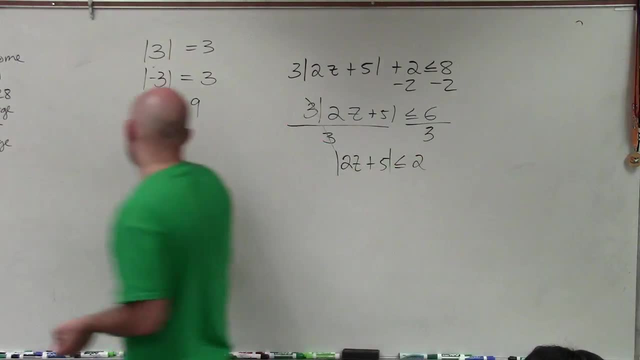 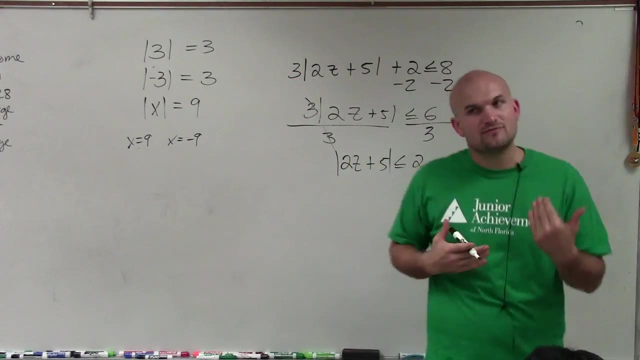 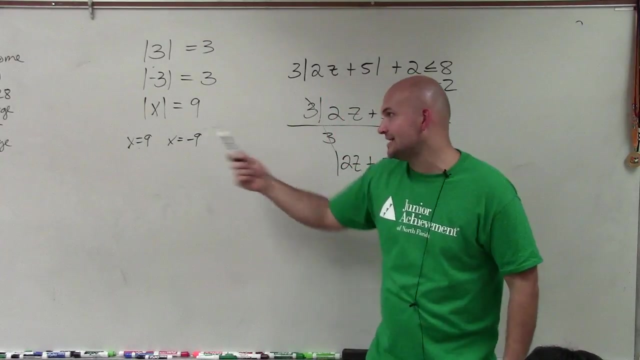 So there's two opportunities You could have: x equals 9 or x equals negative 9.. There's two answers to that. So for absolute value, equations and inequalities, you have to understand we are creating two cases. We need to create the case where, inside, my absolute value is. 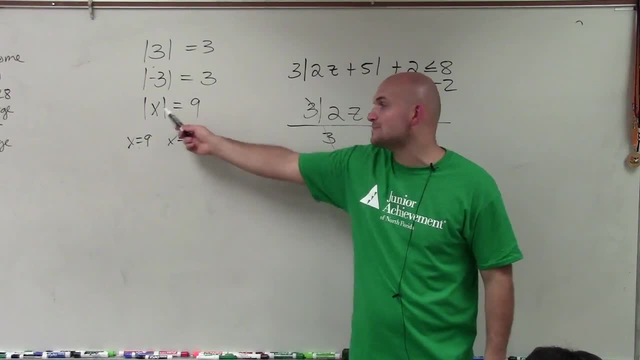 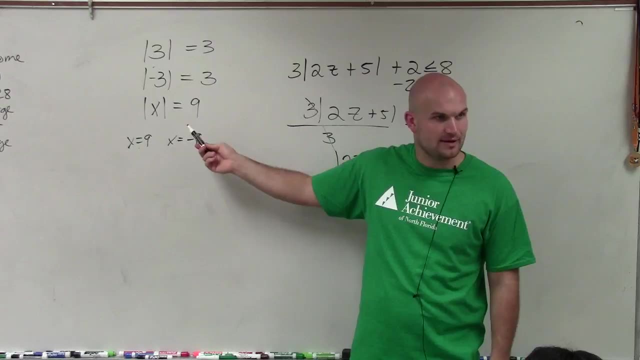 positive And we also need to create the case when, inside, my absolute value is negative, Because it doesn't matter if it's positive or negative 9, it's still going to equal 9.. Yes, Brad, Would we have a problem that some absolute value? 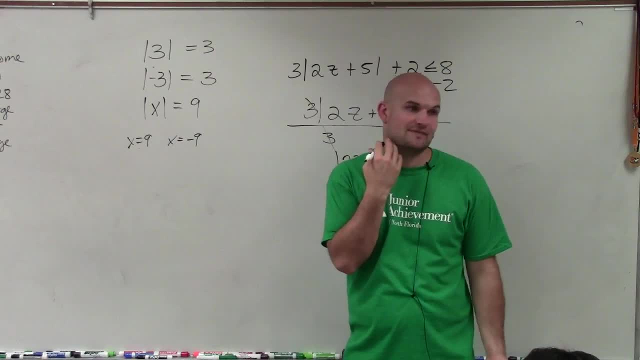 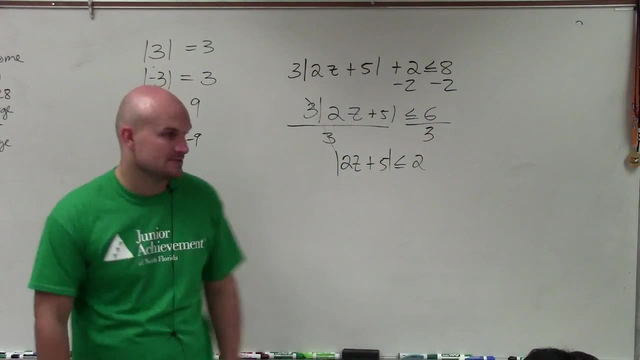 inside of x equals negative 9?. That would be no solution. You can't have that, It's impossible, And there is an example like that on your homework. So what we need to do, ladies and gentlemen, is create two cases. 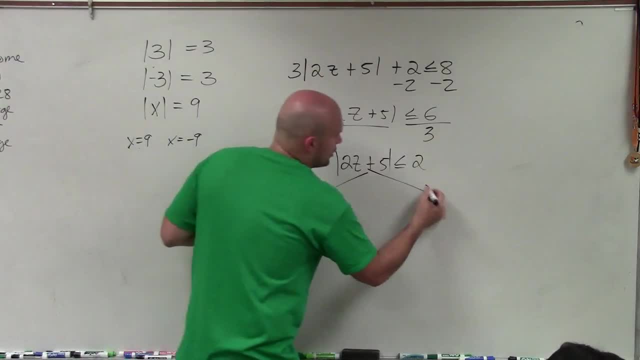 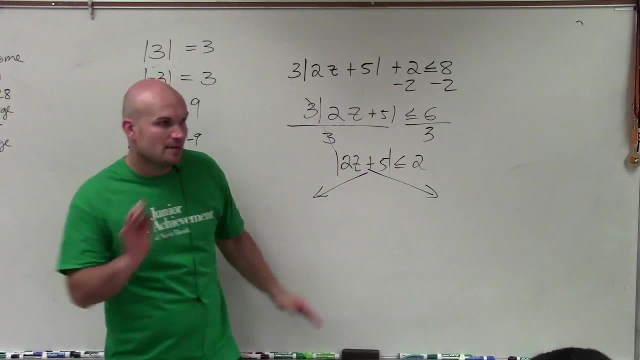 So, if you guys remember, for absolute value equations you can only create two cases once you're absolute, The absolute value is simplified or it's isolated. In this case we have it isolated, But before we create our two cases, I need you guys to understand what are the differences. 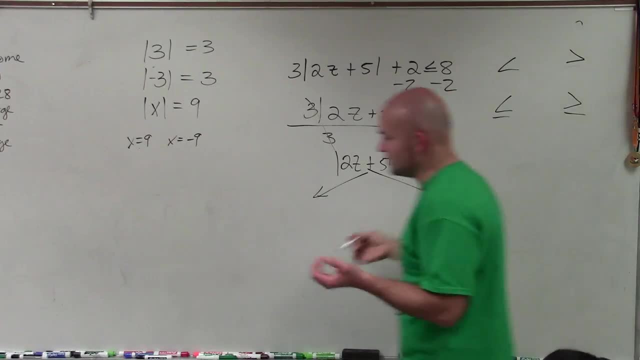 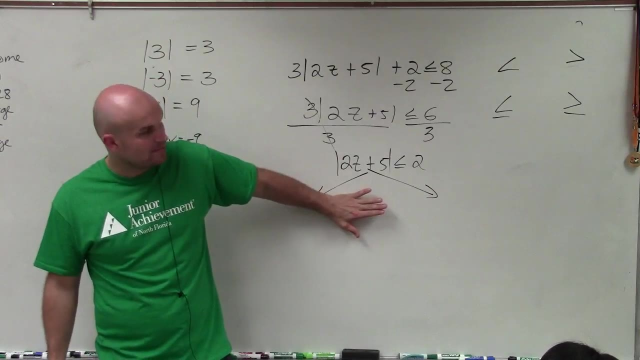 of your two cases. So for absolute value equations, all we did was we set them equally. We set one side, we did the positive and we did the negative. For inequality, it gets a little bit more difficult When we set up our two cases, depending. 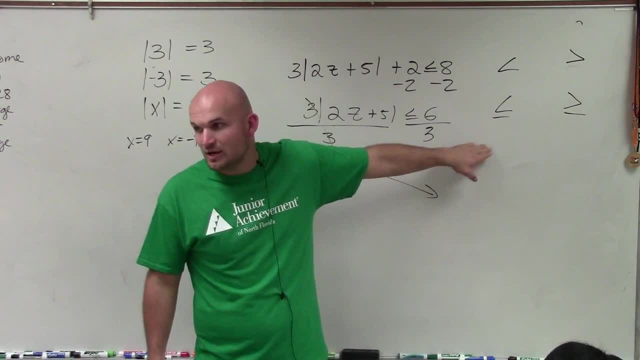 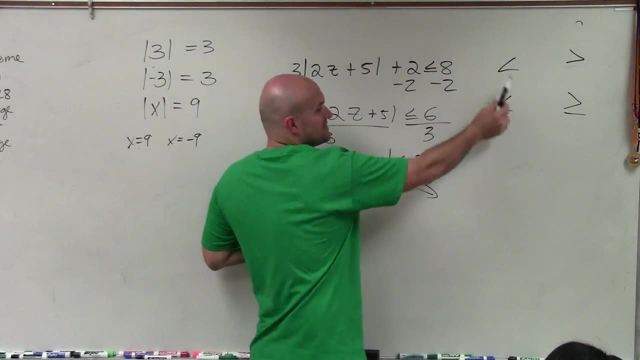 on what your original inequality sign is. that's going to tell you what type of inequality you create, what type of compound inequality you're creating for your two cases. So, if you have a less than, or a less than or equal to, you are now creating an and inequality. 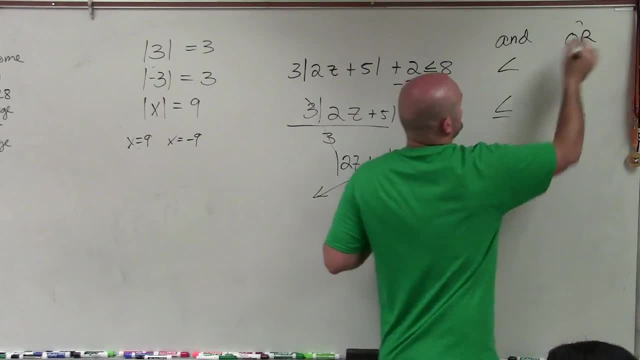 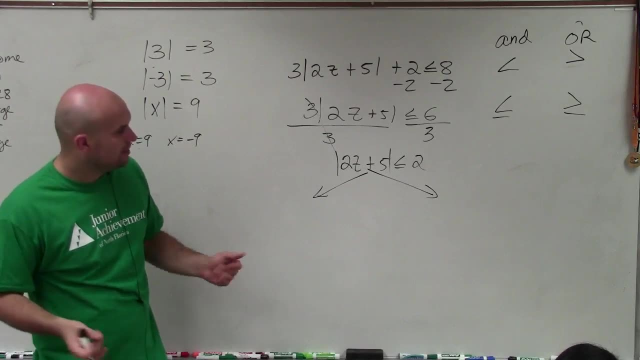 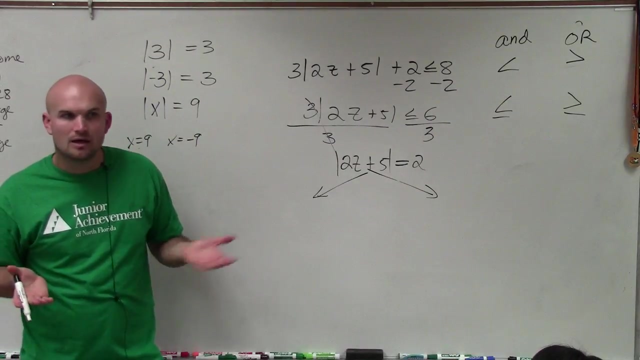 If it's a greater than, or greater than or equal to, you are now creating an or inequality. So what does that mean? Well, ladies and gentlemen, if this wasn't equals, if we were going to do absolute value equations, how would we? 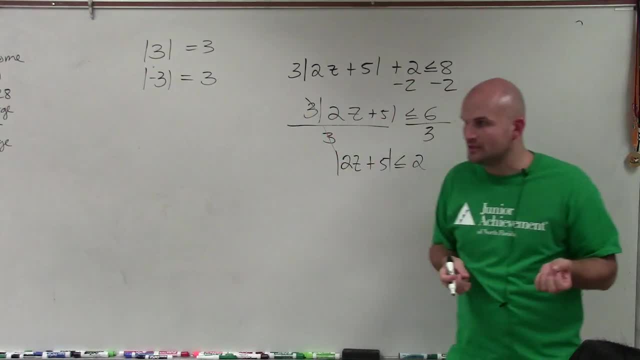 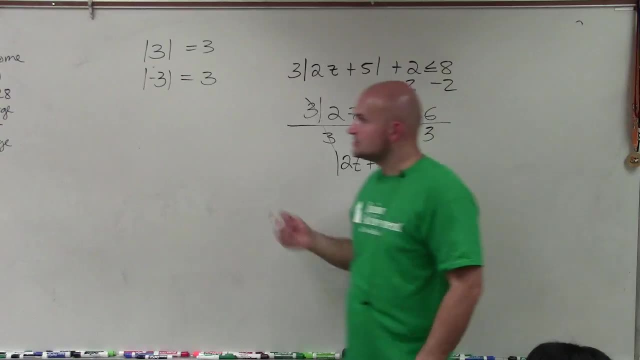 So the absolute distance is always that positive value or the positive distance from, or just the distance from 0, like when you look at the number line. So if I said the absolute value of x is equal to 3,, equal to 9, hopefully you guys can understand. 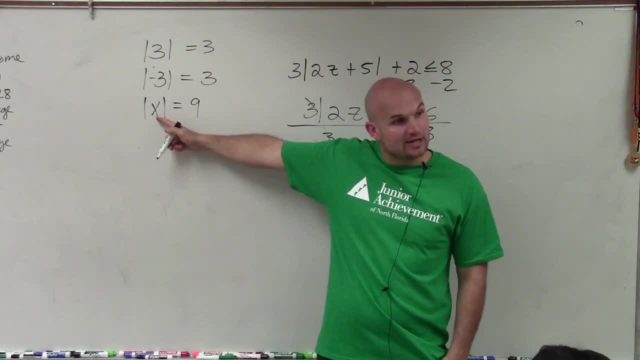 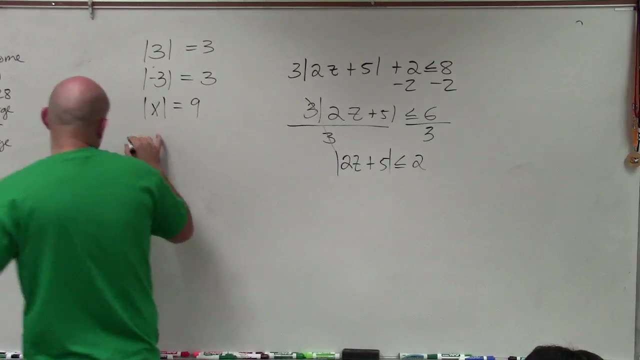 that I could plug in negative 9 in for x, or I can plug in positive 9, correct? Does that make sense? So there's two opportunities. You could have x equals 9 or x equals negative 9.. There's two answers to that. 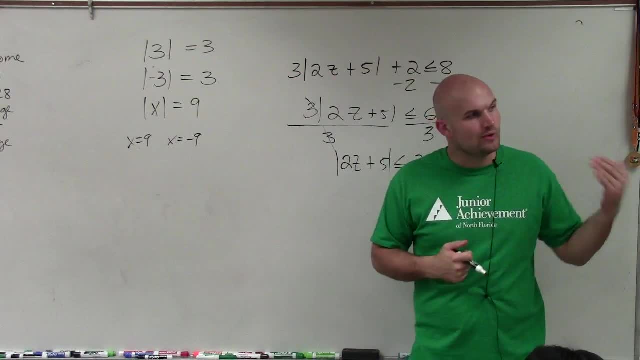 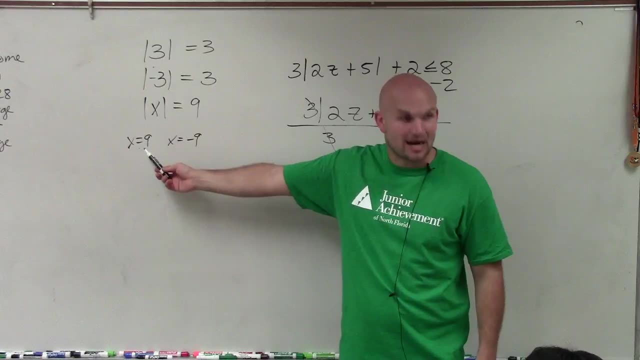 So for absolute value, equations and inequalities, you have to understand we are creating two cases. We need to create the case where, inside, my absolute value is positive, And we also need to create the case when, inside, my absolute value is negative, Because it doesn't matter if it's positive or negative. 9,. 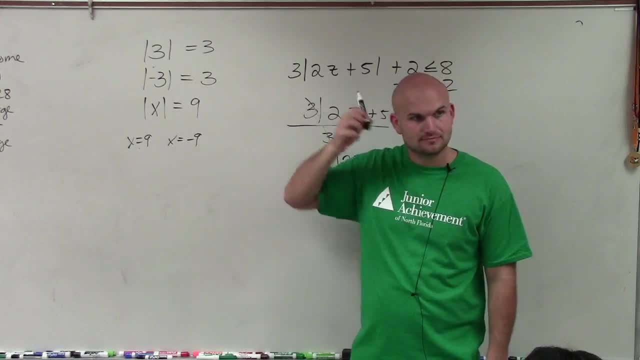 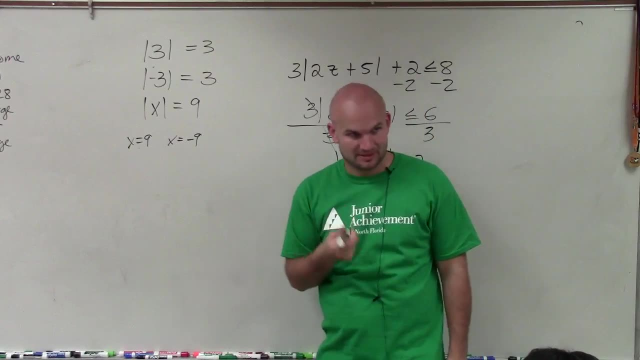 it's still going to equal 9.. Yes, Brad, Would we have a problem that something like absolute value of x equals negative 9? That would be no solution. You can't have that. It's impossible. And there is an example like that on your homework. 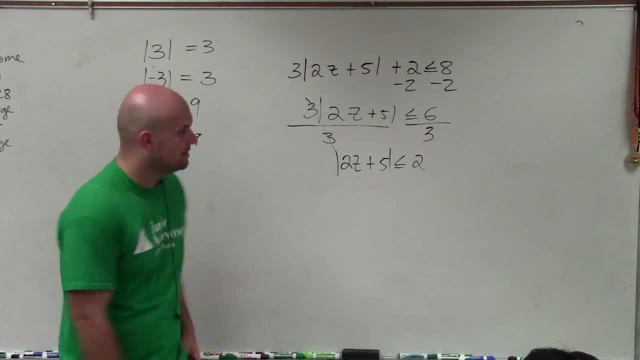 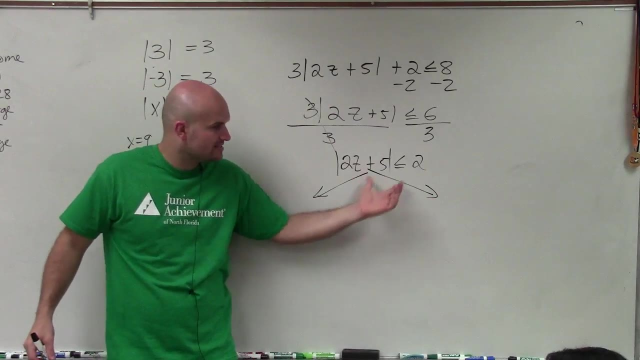 So what we need to do, ladies and gentlemen, is create two cases. So, if you guys remember, for absolute value equations, you can only create two cases once your absolute value is simplified or is it isolated? In this case, we have it isolated. 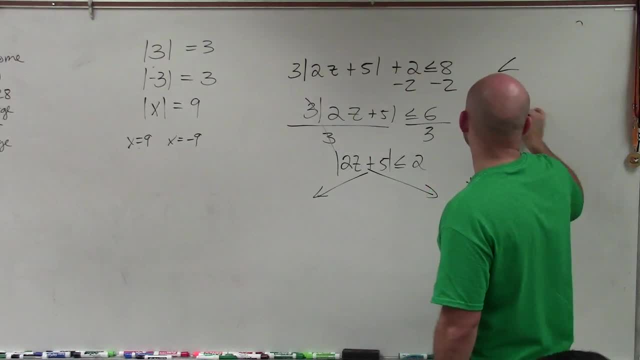 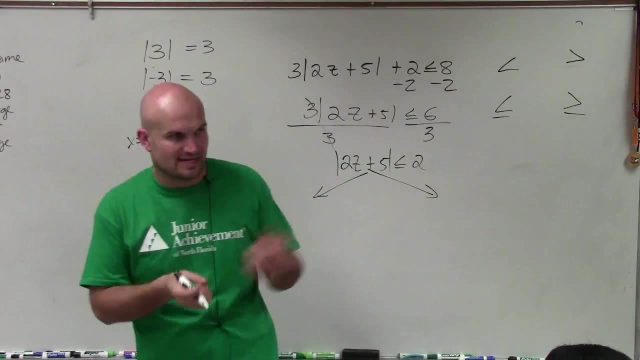 But before we create our two cases, I need you guys to understand what are the differences of your two cases. So, for absolute value equations, all we did was we set them equally, Set one side, we did the positive and we did the negative. 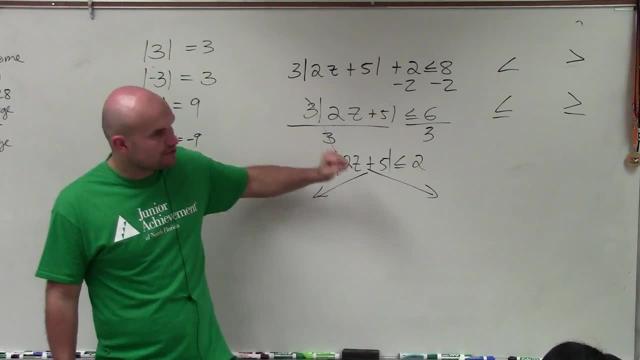 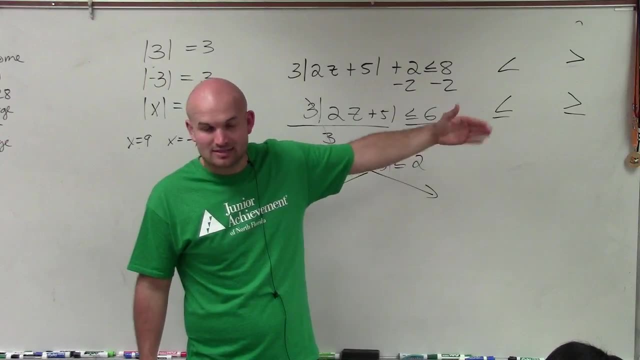 For inequality. it gets a little bit more difficult When we set up our two cases. depending on what your original inequality sign is. that's going to tell you what type of inequality you create, what type of compound inequality you're creating for your two cases. 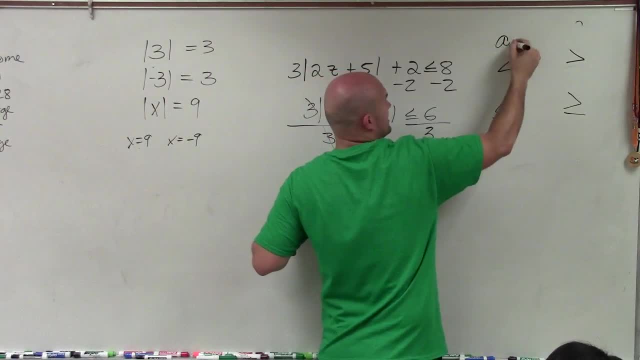 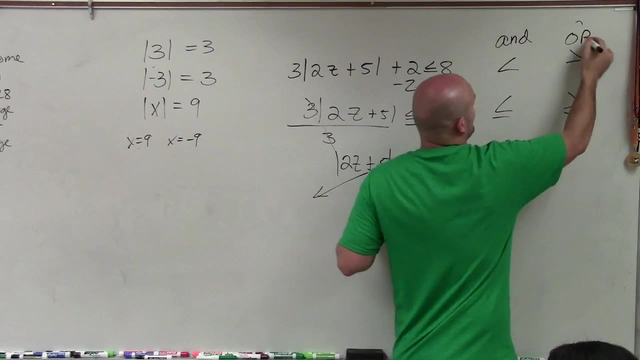 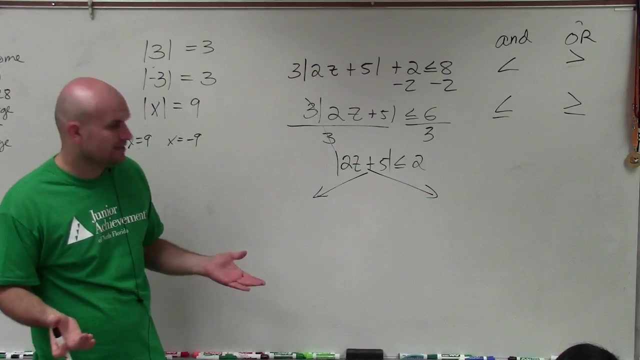 So, if you have a less than, or a less than or equal to, you are now creating an and inequality. If it's a greater than or greater than or equal to, you are now creating an or inequality. So what does that mean? Well, ladies and gentlemen, if this wasn't equals. 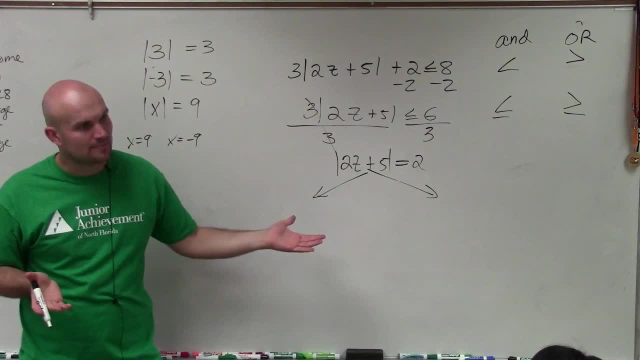 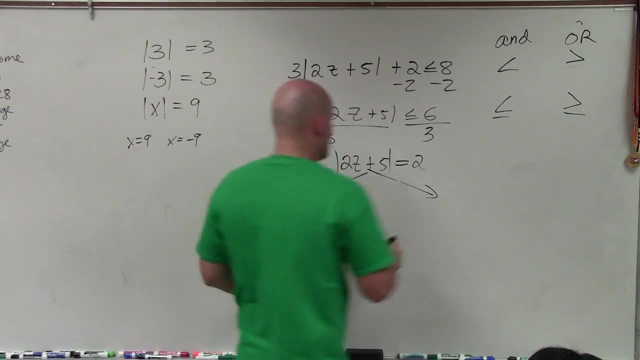 if we were going to do absolute value equations, how would we represent this? We would say: 2z plus 5 is equal to 2.. Notice how I don't need the inequality symbols anymore, or absolute value signs anymore. And then this would be: 2z plus 5 equals negative 2.. 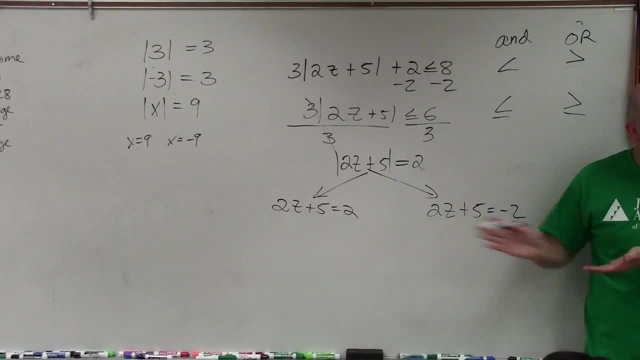 Does everybody agree with me? If we were doing absolute value equations, that's how we would do the two cases: You do one as the positive, or one as it's written, and the other one you negate it. Does that make sense? However, ladies and gentlemen, we don't have an equation. 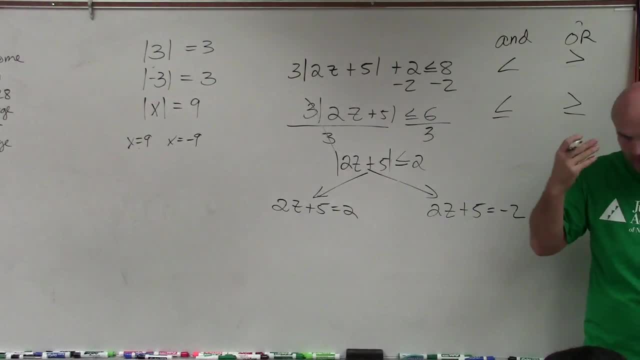 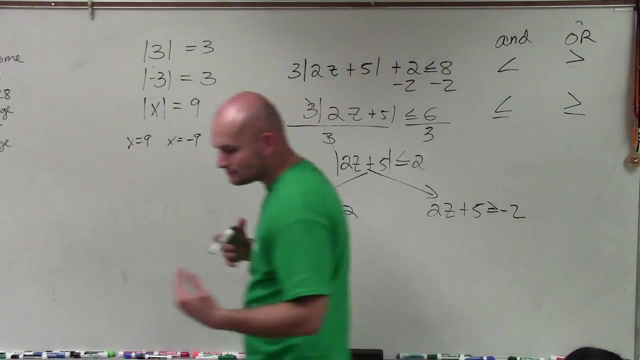 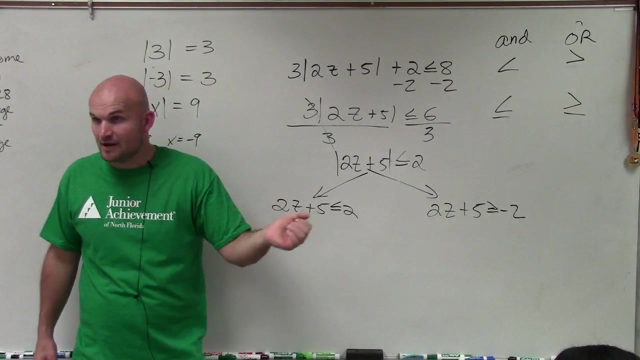 We have an inequality, So when we do our inequality, this remains the same. But now, on the one we negated, we have to flip the sign Because for those of you that are solving one variable inequalities in graphing, you guys remember whenever you multiply or divide by a negative number. 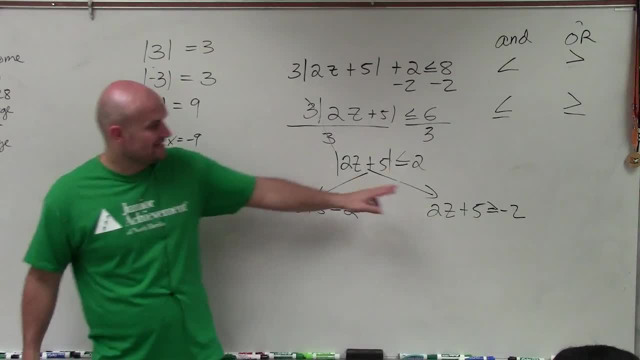 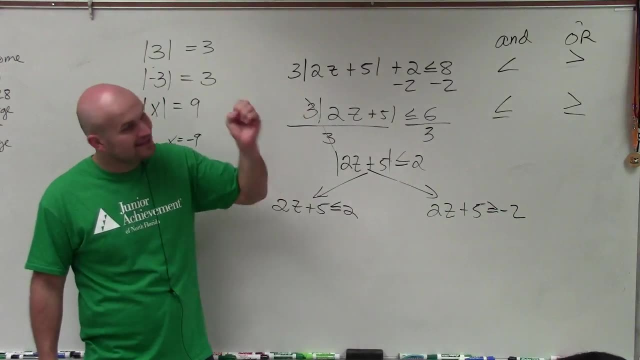 what happens with the sign. You have to flip it right. So if I negate this sign, I've got to, or if I negate the other side, I've got to make sure I flip the inequality sign. The other step is: notice: my original inequality was an and. 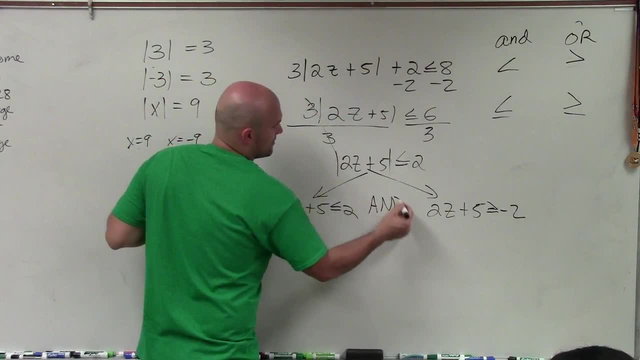 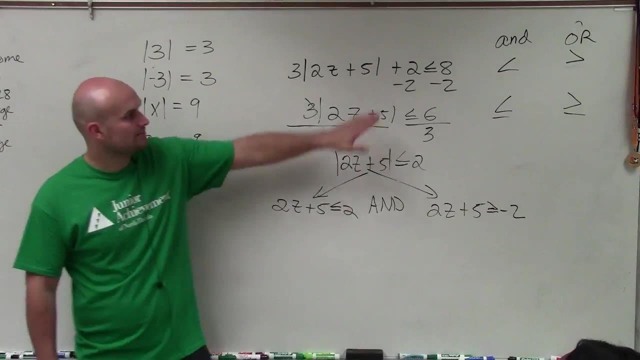 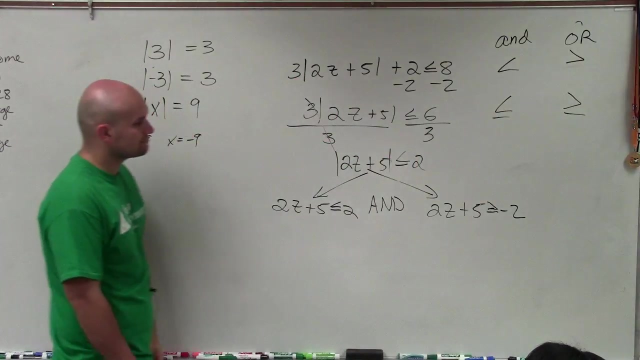 So when I create my two cases, I'm creating a compound inequality of the form and because that's with my original inequality. So it's going to be very important you guys know the distinction between these two for your absolute value. Now, is it OK if you guys solve for these? 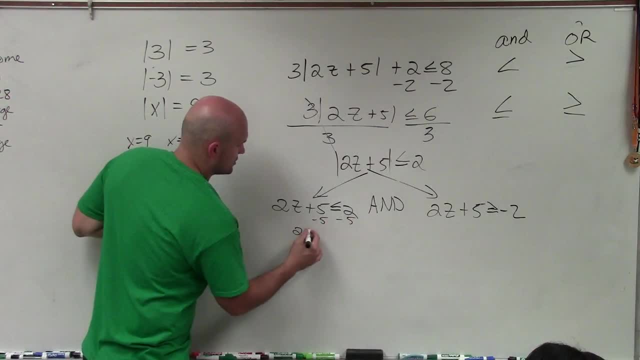 Yeah, So we can solve. So 2z is less than or equal to a negative 3. Divide by 2, divide by 2.. z is less than or equal to a negative. 3 halves Over here, minus 5, minus 5.. 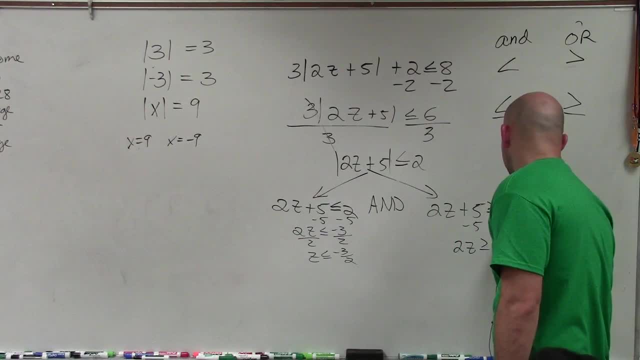 2z is greater than or equal to minus 5.. So that would be a negative 3.. Divide by 2, divide by 2.. Wait a minute, What did I do? What did I do wrong? Oh, it's negative 7.. 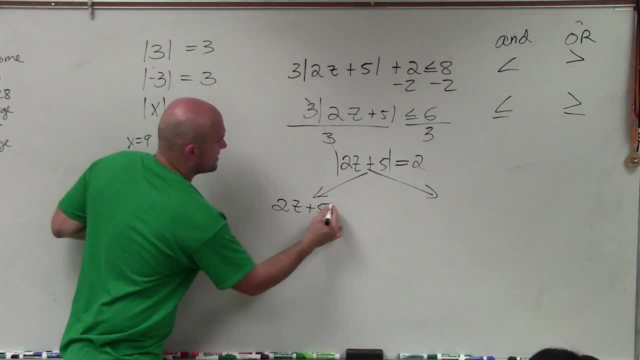 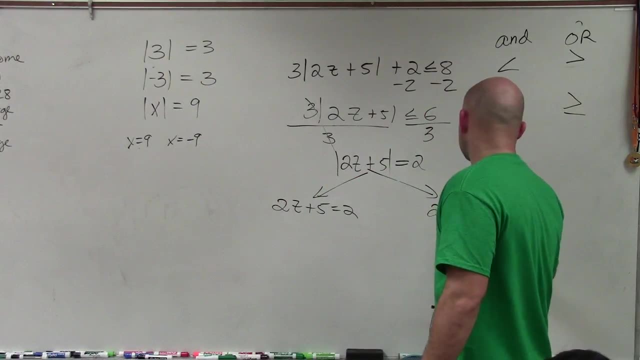 represent this. We would say: 2z plus 5 is equal to 2.. Notice how I don't need the inequality symbols anymore, or absolute value signs anymore. And then this would be: 2z plus 5 equals negative 2.. Does everybody agree with me? 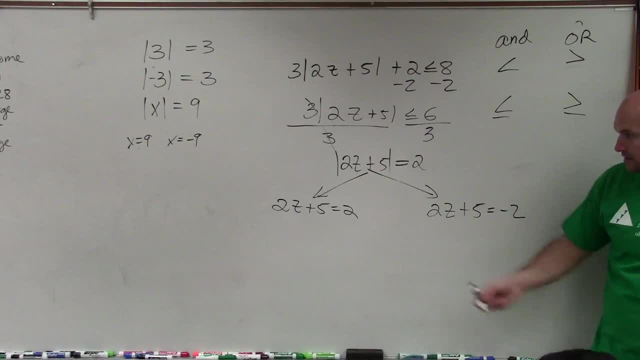 If we were doing absolute value equations, that's how we would do the two cases: You do one as the positive, or one as it's written, and the other one you negate it. Does that make sense? However, ladies and gentlemen, we don't have an equation. 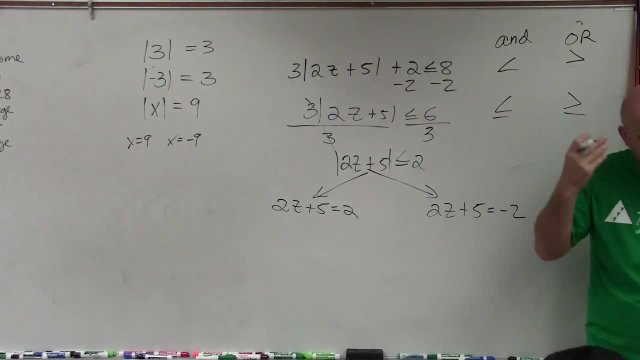 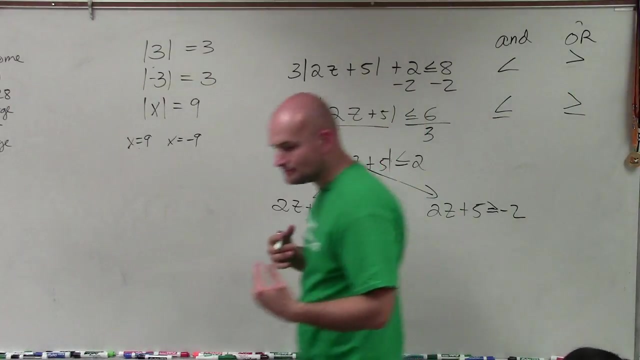 We have an inequality, So when we do our inequality, this remains the same. But now, on the one we negated, we have to flip the sign, Because for those of you that are solving one variable inequalities in graphing, you guys, 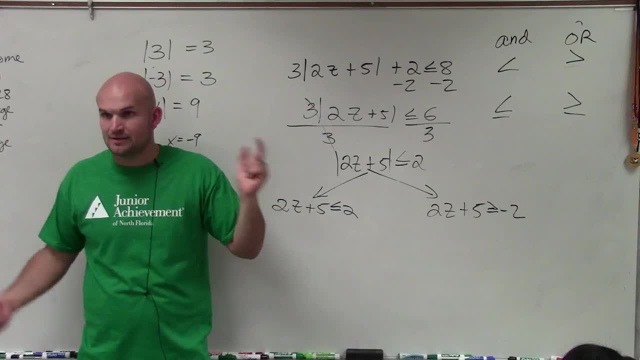 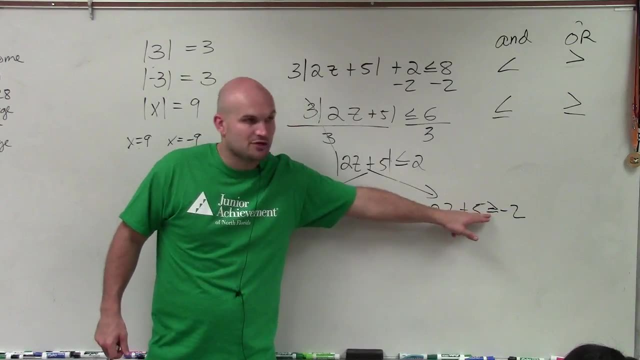 remember, whenever you multiply or divide by a negative number, what happens with the sign? You have to flip it right. So if I negate this sign, I got them. or if I negate the other side, I got to make sure I flip the inequality sign. 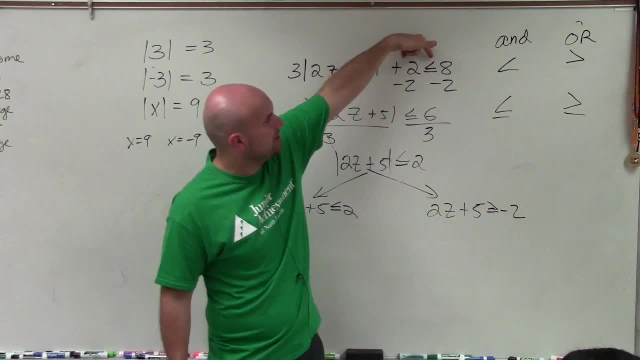 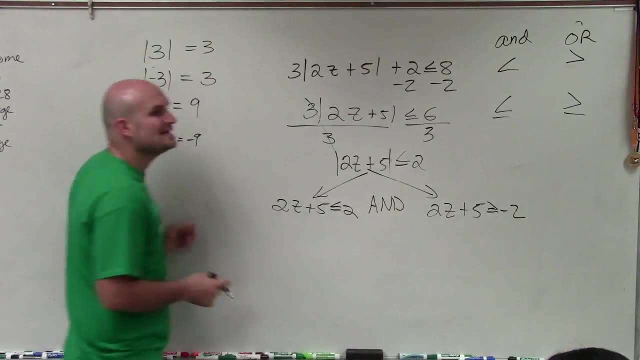 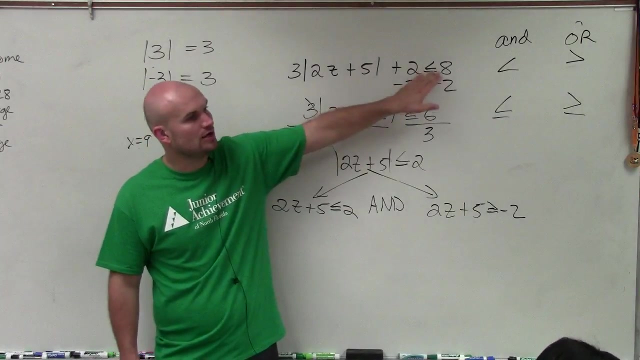 The other step is: notice: my original inequality was an and. So when I create my two cases, I'm creating a compound inequality of the form and because that's with my original inequality. So it's going to be very important, you guys know. 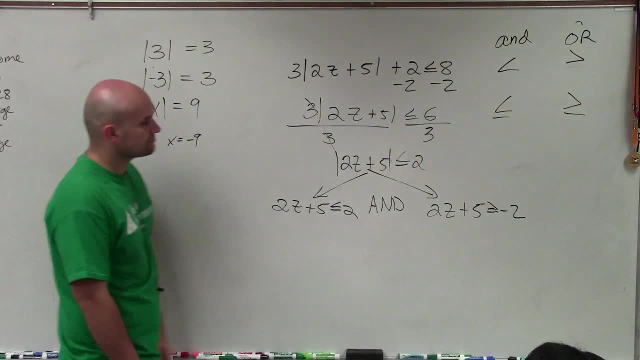 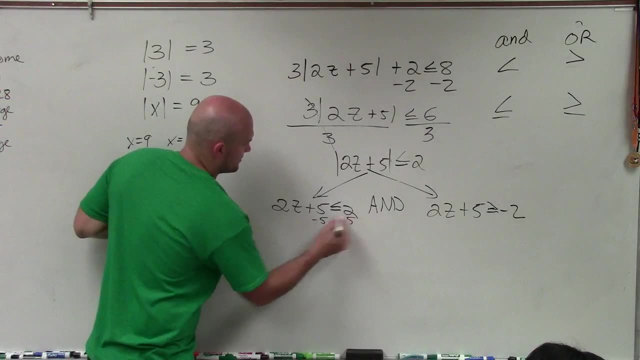 the distinction between these two for your absolute value. Is it OK if you guys solve for these? Yeah, So we can solve. So 2z is less than or equal to a negative 3.. Divide by 2.. Divide by 2.. 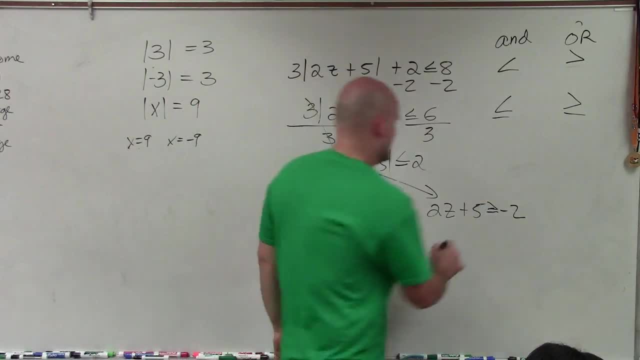 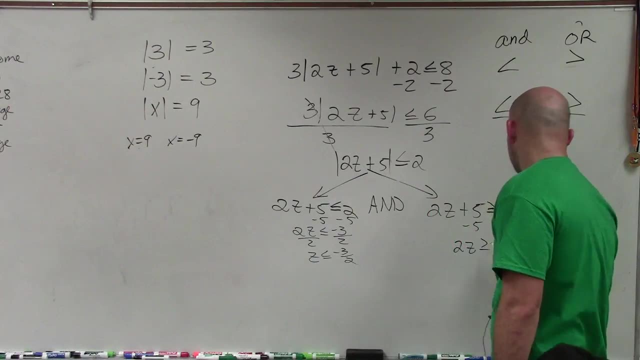 z is less than, or equal to a negative 3 halves Over here- minus 5,, minus 5.. 2z is greater than or equal to minus 5. So that would be a negative 3.. Divide by 2.. 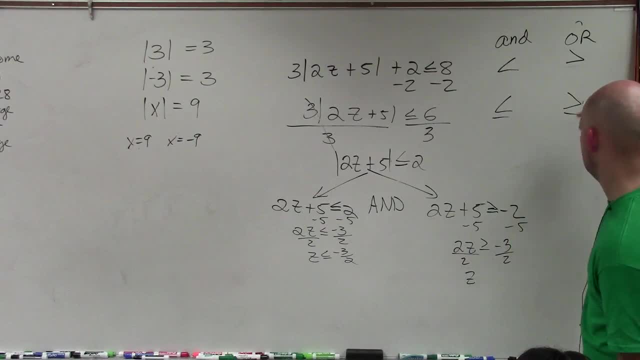 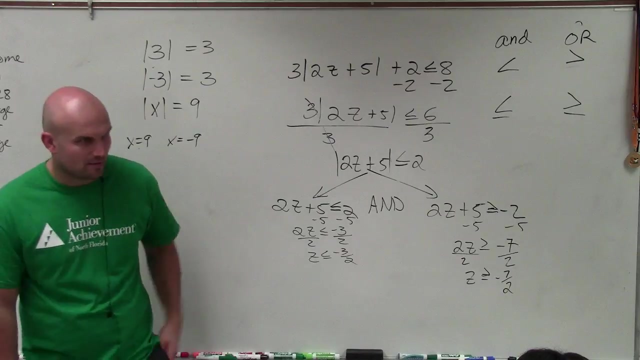 Divide by 2.. Wait a minute. What did I do wrong? Oh, it's negative 7.. No wonder. So I really don't like using decimals, But when I'm graphing I think decimals sometimes are easy to understand. how to graph? 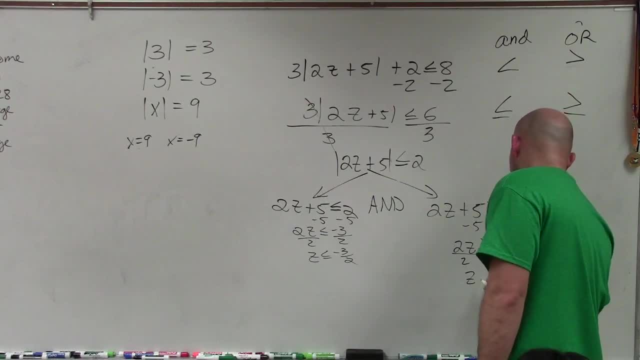 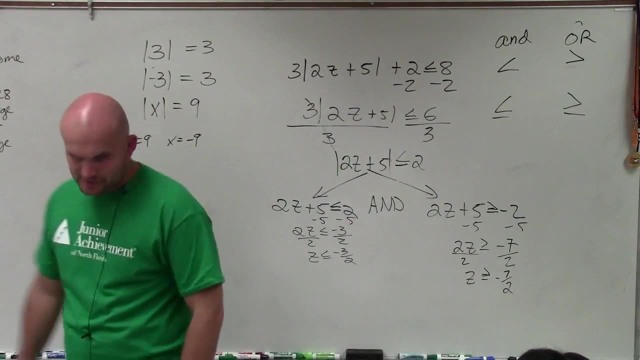 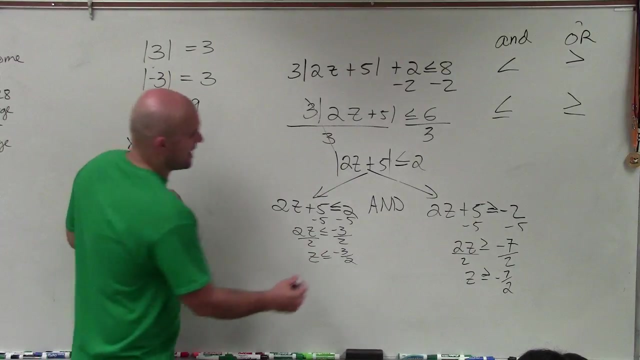 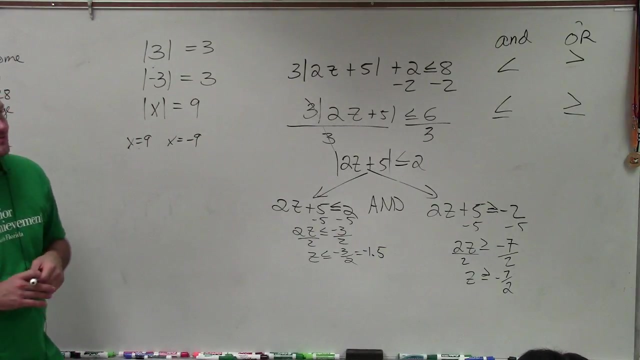 No wonder. So I really don't like using decimals, But when I'm graphing I think decimals sometimes are easy to understand how to graph. So negative 3 halves is equal to negative 1.5.. And negative 7 halves. 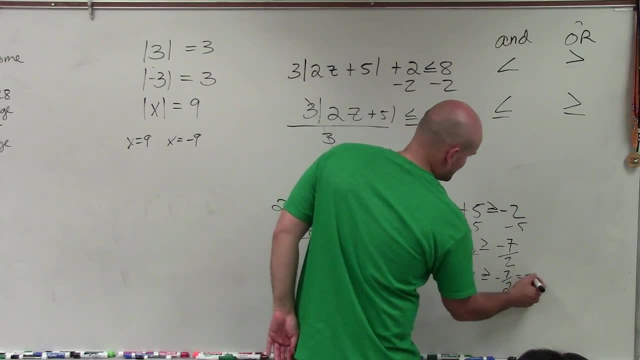 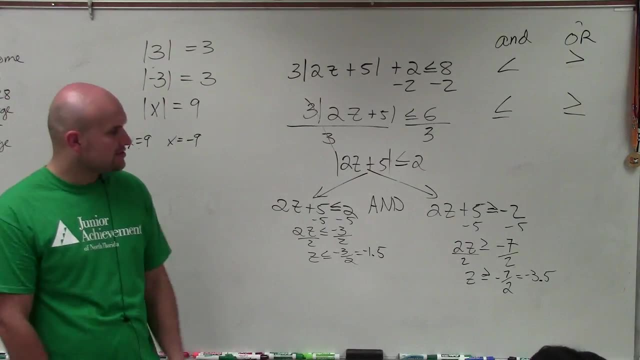 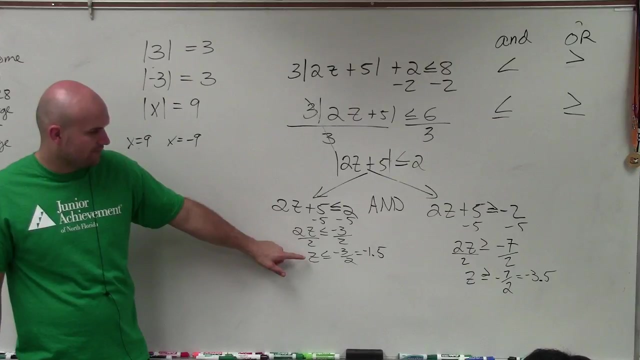 And negative 7 halves is equivalent to negative 3.5.. If you guys want to use your calculator, that's fine to go into there. So basically, ladies and gentlemen, what I have is y is less than negative 1.5.. 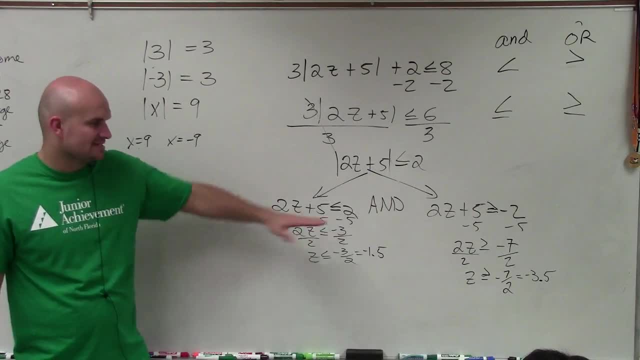 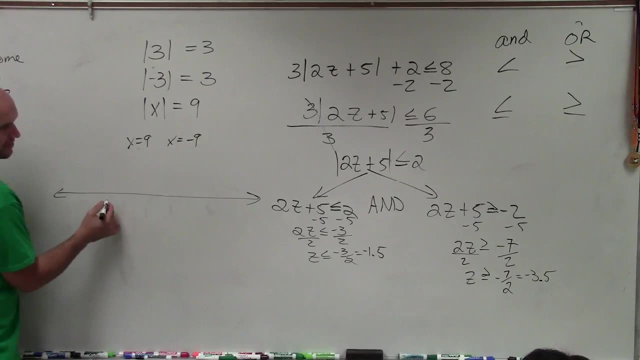 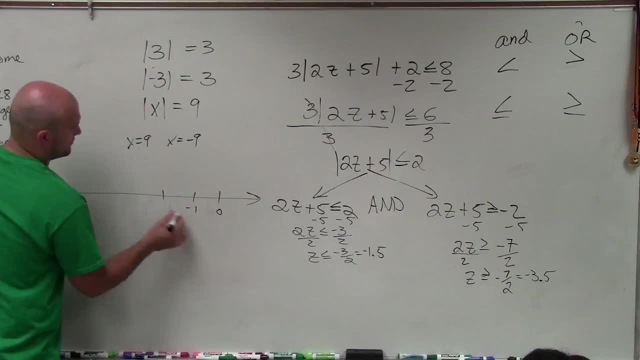 Let's have 0 here, Negative 1, negative 2, negative 3, negative 4, negative 5.. And here's positive 1.. So what we need to do when we're doing an? and does anybody remember what an and what's? 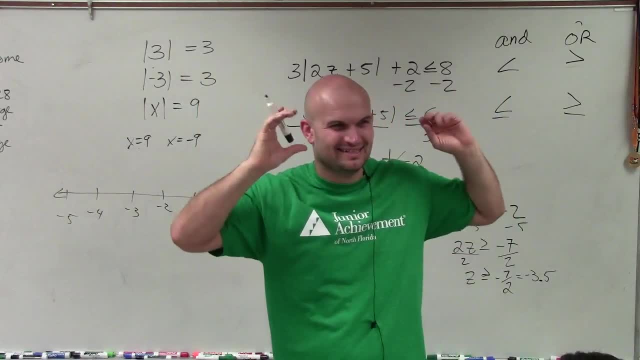 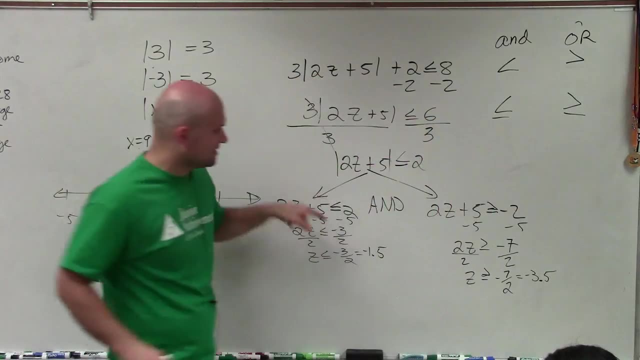 important about graphing an? and Anybody want to raise their hand. What's important about graphing an? and There's something that's very, very important- Yes, Well, that's going to deal with the inequality symbol. Well, what are we looking for when we're graphing an? and? 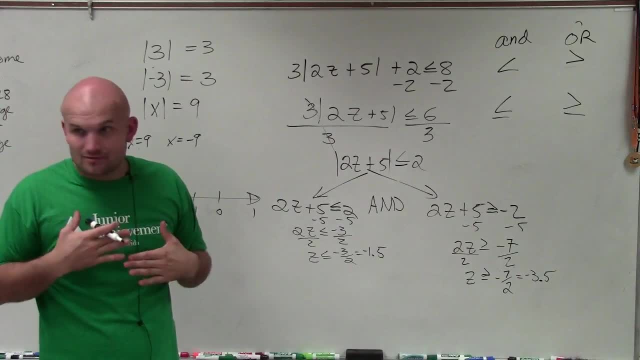 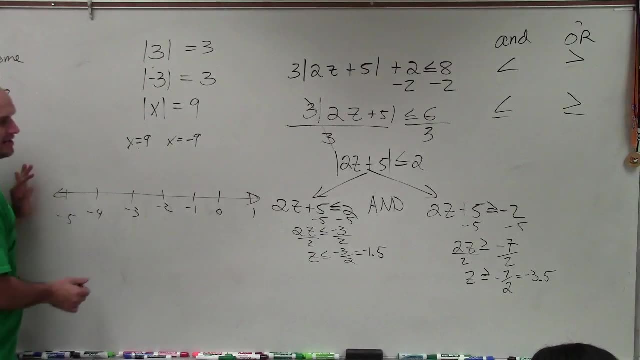 compound inequality. We're looking for the intersection right And is where they intersect. So what we have to do is we have to graph each of these separately. all right, So to graph: z is less than negative 1.5, I estimate where 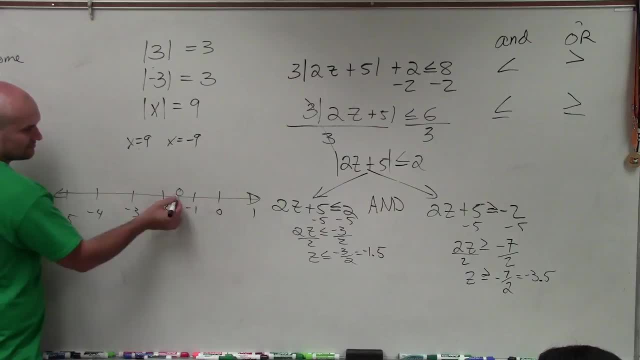 negative 1.5 is which is like right here, right, So I'll put a nice little dot Now all the values that are less than negative 1.5, is that going to be going to the left or to the right? 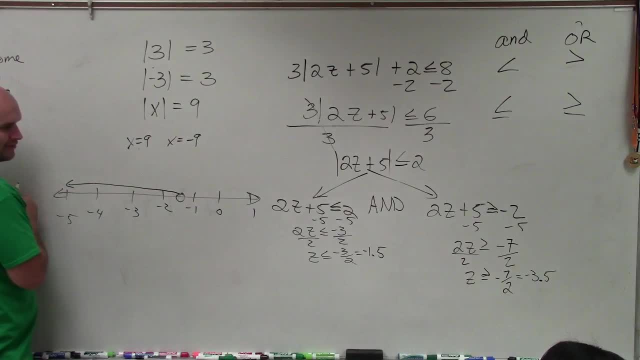 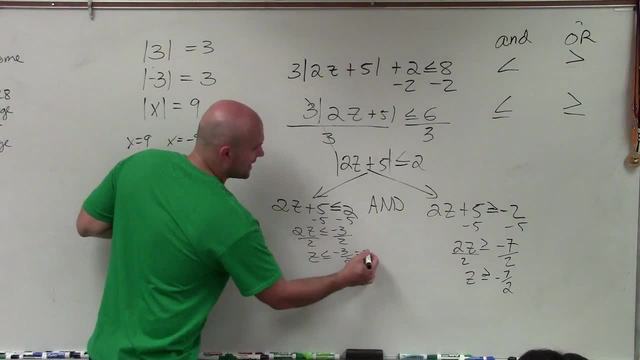 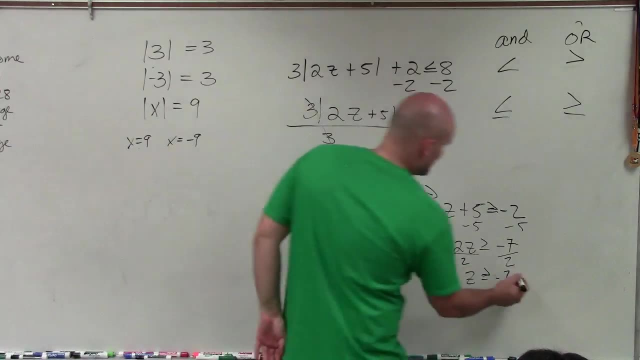 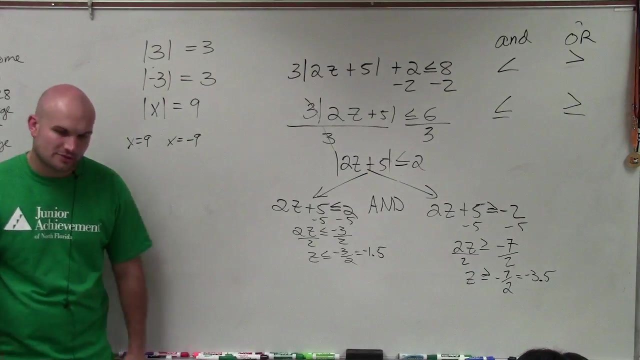 So negative 3 halves is equal to negative 1.5.. And negative 7 halves Is equivalent to negative 3.5.. If you guys want to use your calculator, that's fine to go into there. So basically, ladies and gentlemen, what I have is y. 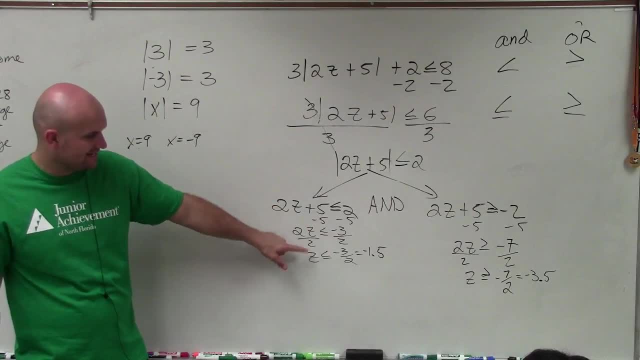 is less than negative 1.5 and z is less than negative 1.5 and z is greater than negative 3.5.. So how are we going to look? How is that going to look? So let's do, Let's have a look. 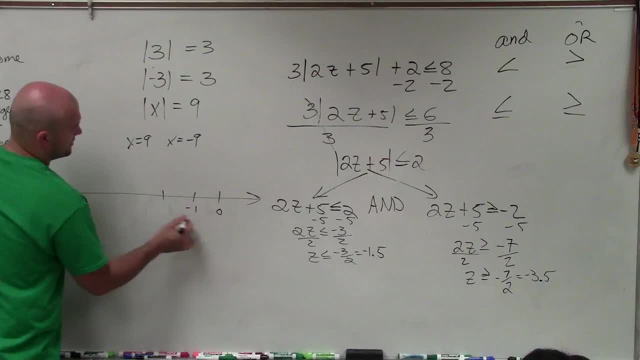 Let's have 0 here, Negative 1, negative 2, negative 3, negative 4, negative 5.. And here's positive 1.. So what we need to do when we're doing an? and does anybody remember what an and what's? 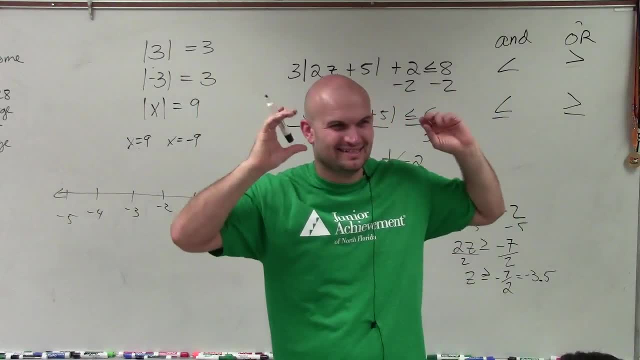 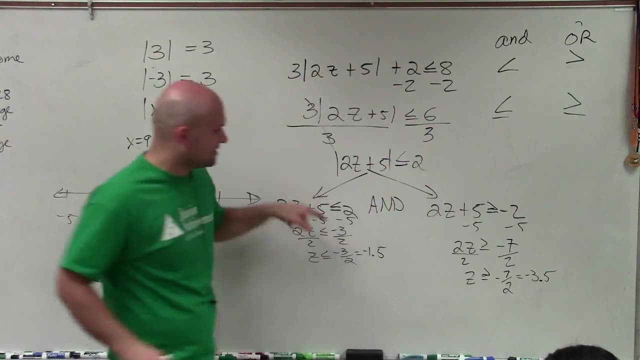 important about graphing an? and Anybody want to raise their hand. What's important about graphing an? and There's something that's very, very important- Yes, Well, that's going to deal with the inequality symbol. Well, what are we looking for when we're graphing an? and? 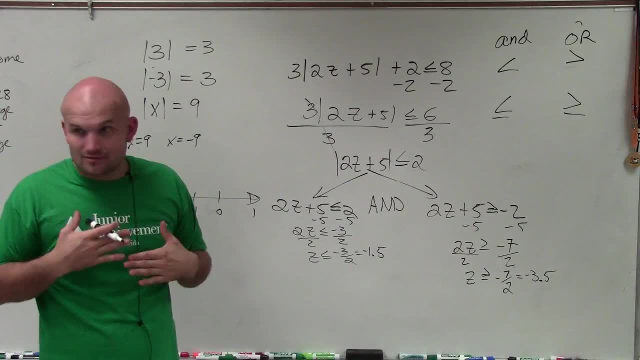 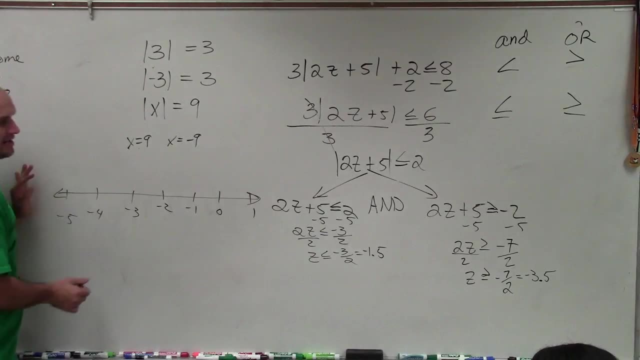 compound inequality. We're looking for the intersection right And is where they intersect. So what we have to do is we have to graph each of these separately. So to graph z is less than negative 1.5, I estimate where negative 1.5 is, which is like right here. 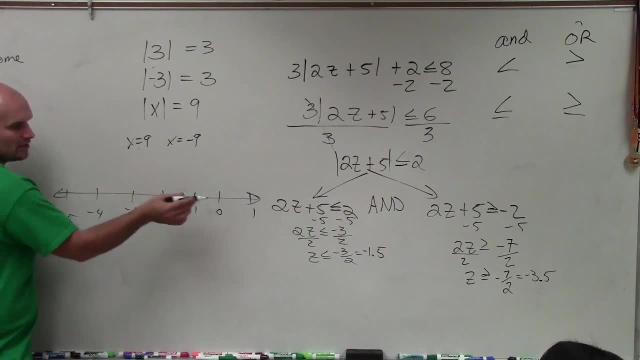 So I'll put a nice little dot Now. all the values that are less than negative 1.5,. is that going to be going to the left or to the right? To the left, Everybody agree? Yes, Everybody agree with me. that's what that would look like. 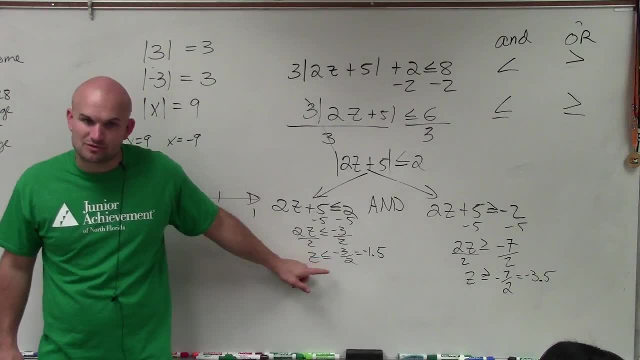 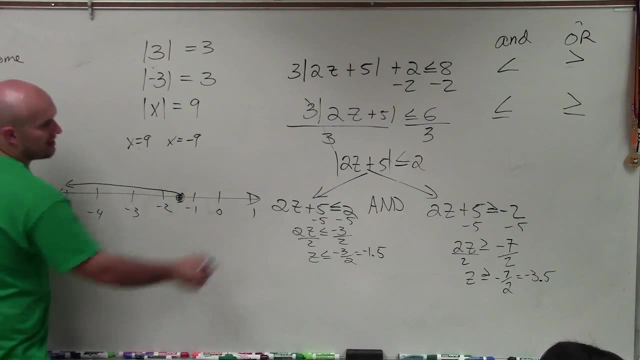 Oh, and then, going back to Brianna's comment, this is less than or equal to, So is that going to be shaded in or open? It's going to be closed right Now, let's go, and graph z is greater than negative 3.5.. 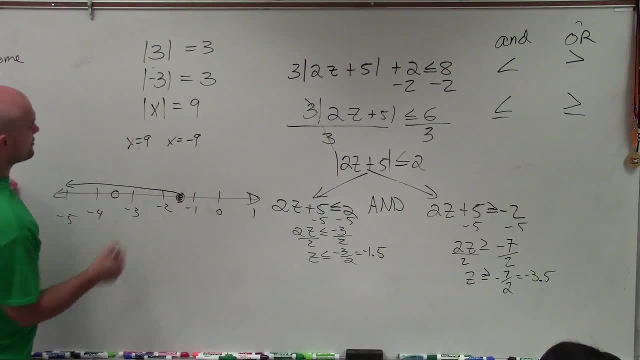 So I go and find negative 3.5, which is right here Again, that's greater than or equal to. so that's going to be open And then that one says all values that are greater than negative 3.5.. 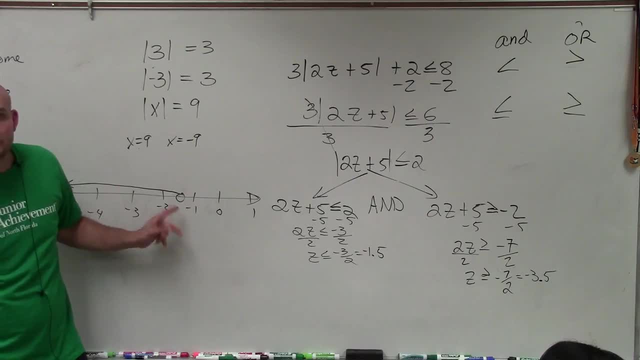 So is that going to be shaded in or open? It's going to be closed. right Now let's go and graph z is greater than negative 3.5.. So I go and find negative 3.5, which is right here.